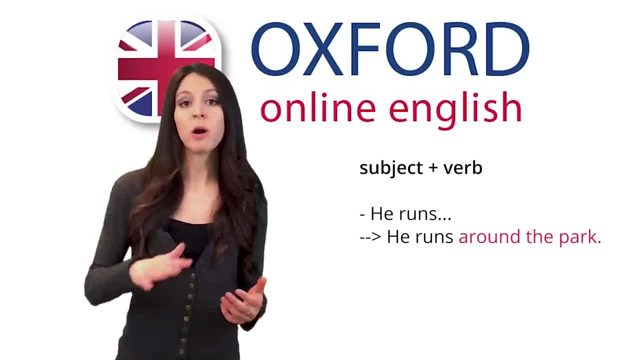 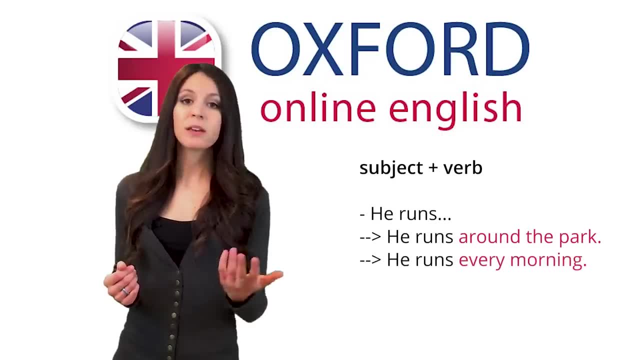 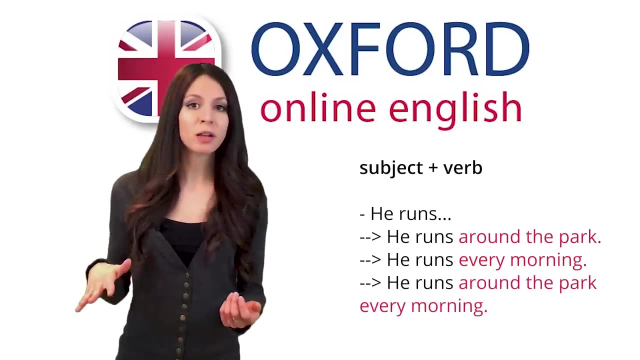 He runs slowly. You can also add an adverb of place. He runs all around the park. What better adverb could you have? You could add an adverb of time. He runs every morning. You could add both. He runs around the park every morning. 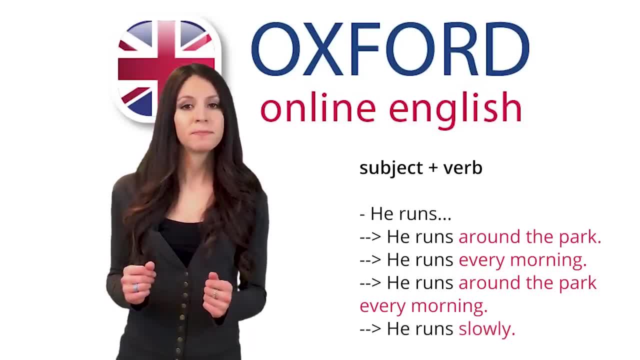 You could add an adverb of manner: He runs slowly. many choices, but your choices are also limited. In this case. you can use different kinds of adverbs, but there are also things you can't use. For example, you can't use another verb after run. 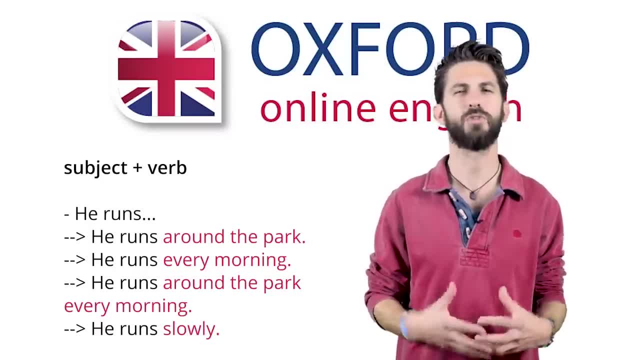 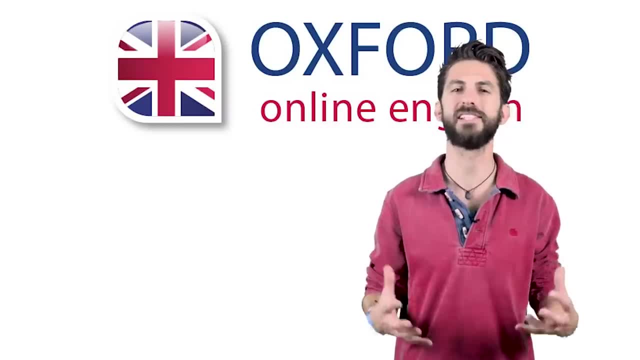 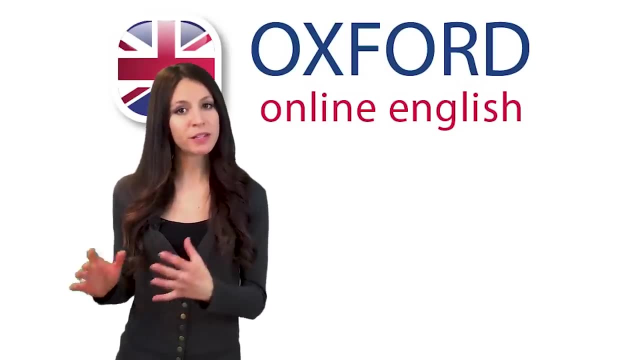 You can't use an adjective, You can't use a noun, or at least you can't use a noun with this meaning of run. This is an important point. Let's look at it in more detail To build grammatically complete sentences in English. there's one important question. 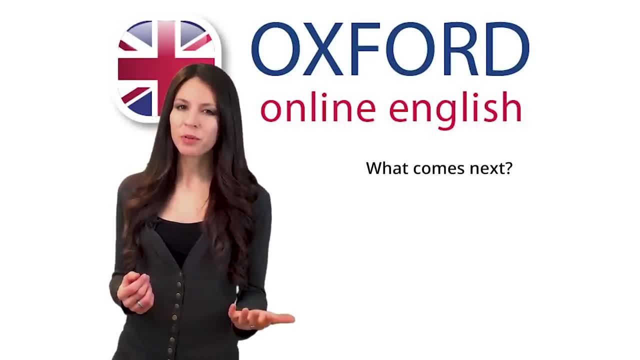 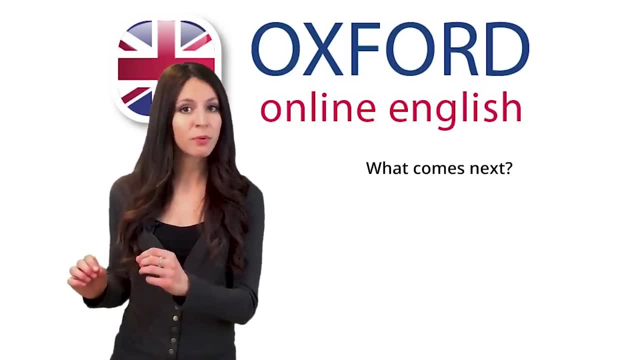 What needs to come next. For example, you saw the sentence he runs. That's a complete sentence. You can put a full stop after runs, and it's correct. It's very basic, but it's correct. What about these? 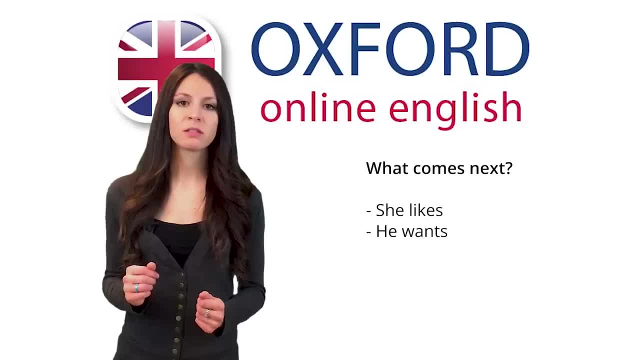 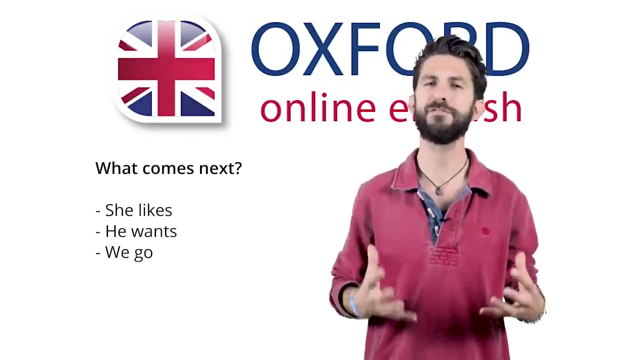 She likes, He wants, We go. These aren't complete sentences. Can you explain why not They aren't complete? very simply because they aren't finished. Look at the first sentence: she likes. She likes what She has to like, something. 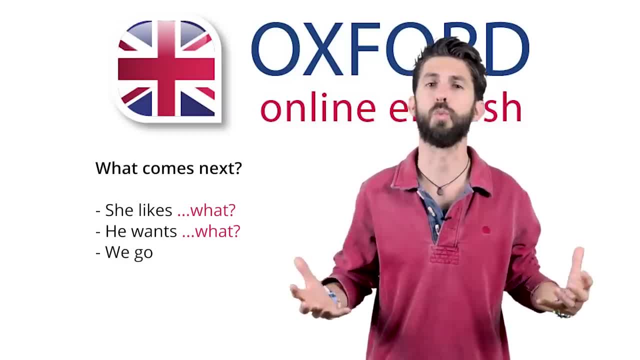 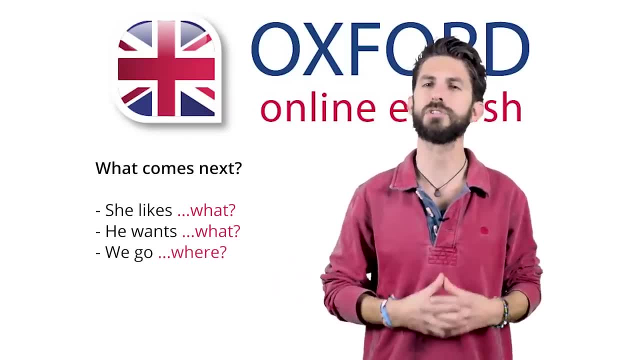 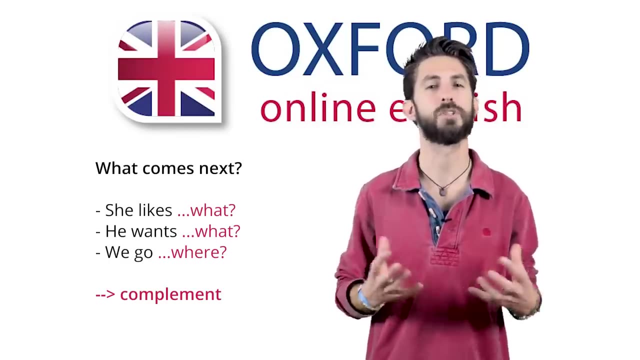 He wants? What does he want? You can't just want, You have to want something. We go Where? At this point? we want to teach you a word, a complement. The complement is the thing you add after a verb to make a sentence complete. 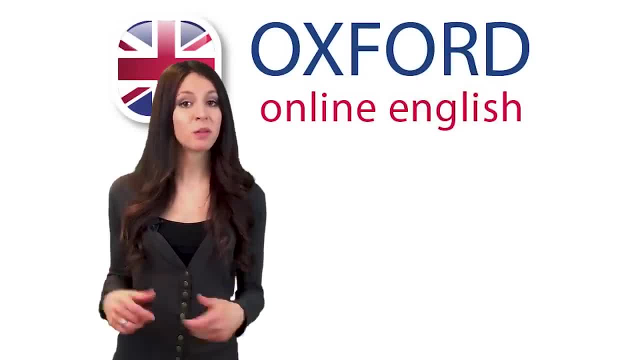 A complement can have many different forms. It can be a noun, a verb, an adjective or an adverb. These things can be single words or phrases, For example…. For example, when we say noun, we also mean noun phrases. 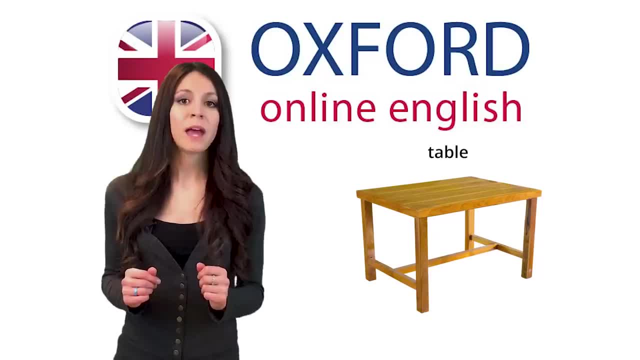 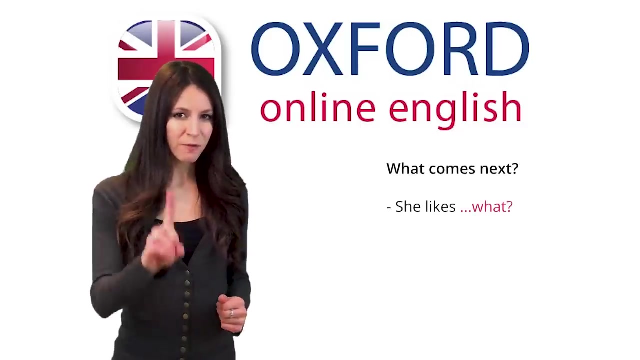 So table is a noun And the wooden table which my grandmother gave me is also a noun. Both nouns refer to one object, one table. For this lesson, a noun can be one word or a phrase. Okay, Let's practice. Look at the first sentence. 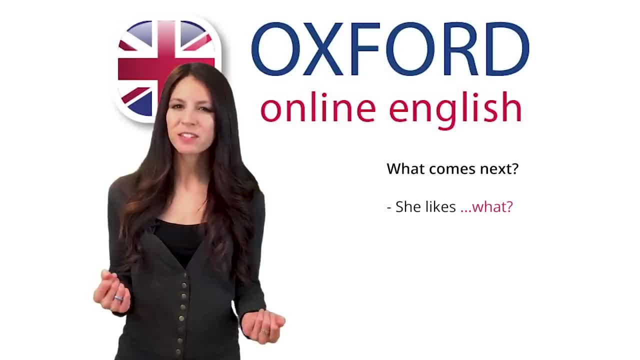 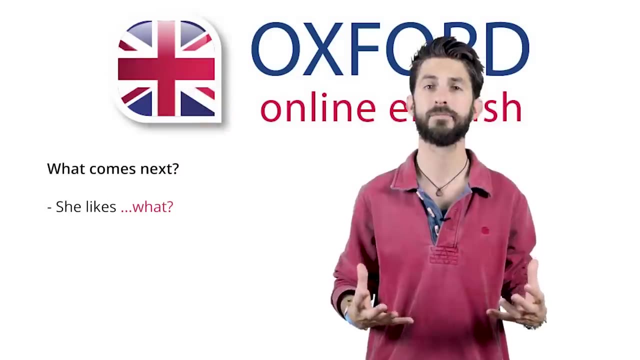 She likes. How could you finish this? What are the possible complements? Pause the video and write down three endings for your sentence. Try to use different ideas and structures. Ready, Let's look at some possible answers. These are just our suggestions. 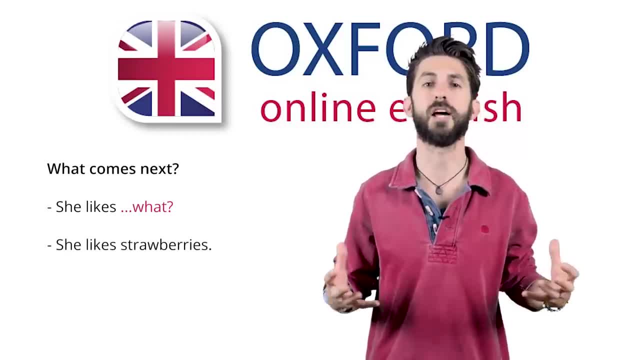 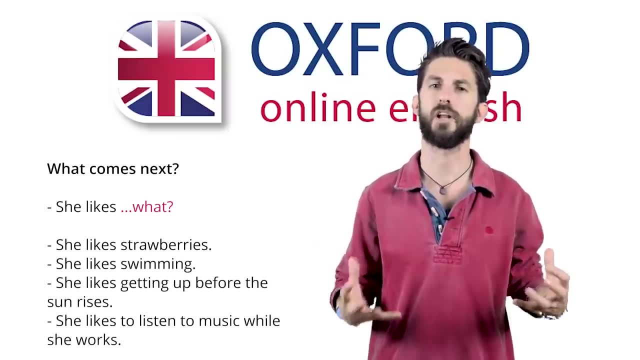 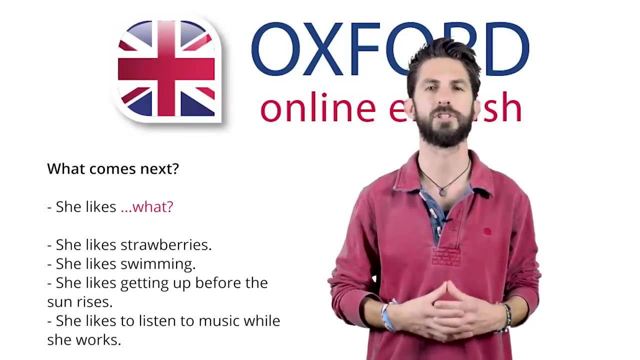 Of course, there are many possibilities. Ready, She likes strawberries, She likes swimming, She likes getting up before the sun rises, She likes to listen to music while she works. You can see that there's more than one possible complement. You can use a noun, a gerund, with a verb ing which acts like a noun, a gerund phrase. 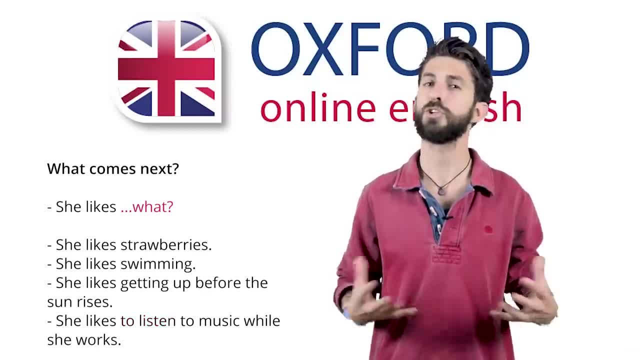 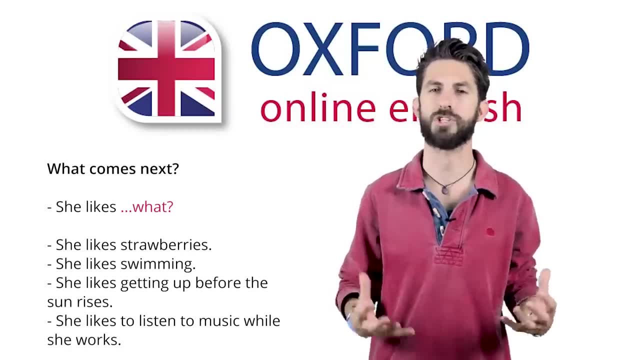 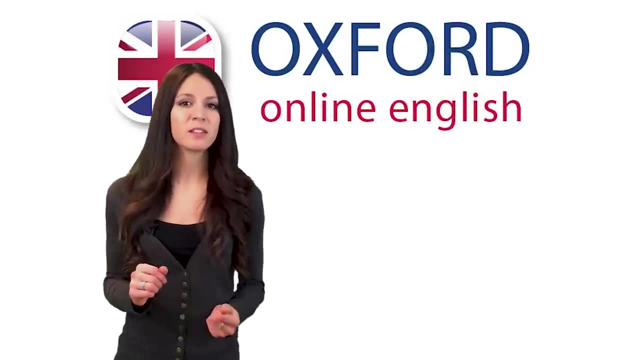 or an infinitive verb with to. So you have many choices. However, Like before, Voices are also limited. Only certain structures are possible. The idea of complements isn't just for the first verb in the sentence. Many words need a complement. 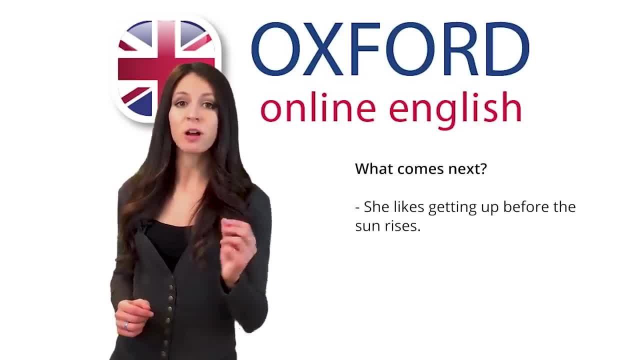 For example, look at one of the sentences you just saw: She likes getting up before the sun rises. Technically you can say she likes getting up. It's a grammatically complete sentence: She likes getting up before the sun rises. 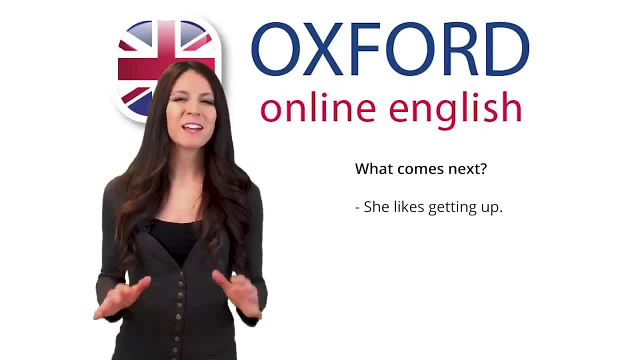 She likes getting up. There are more than one possible complement, Not sure which right. It doesn't make any sense. You need more information. She likes getting up When, Why, How. You need a complement after getting up to complete the idea. 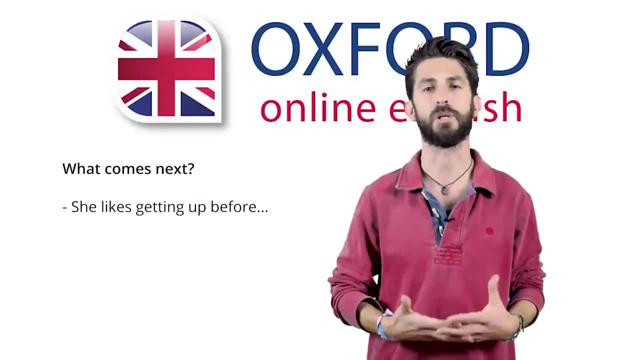 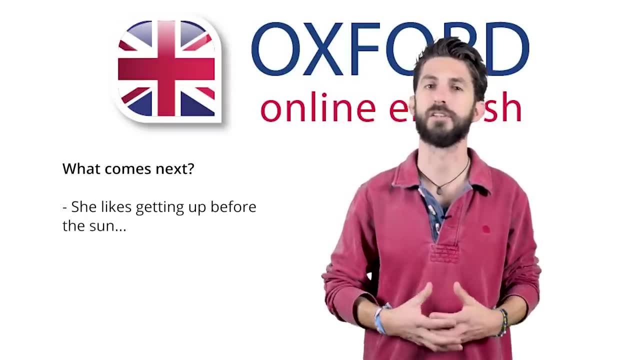 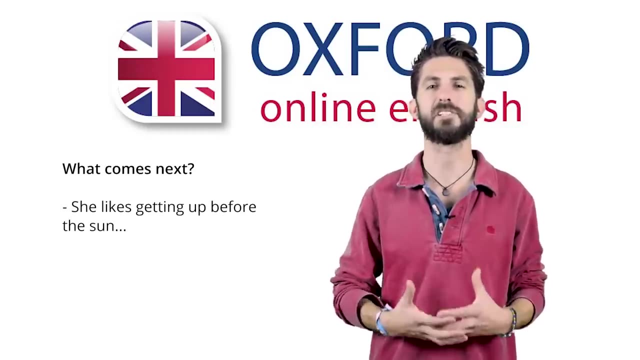 She likes getting up before the sun rises Before also needs a complement. You can't stop there Before what She likes- getting up before the sun. This also doesn't work because it doesn't make sense. It doesn't make sense because the sun needs a complement. 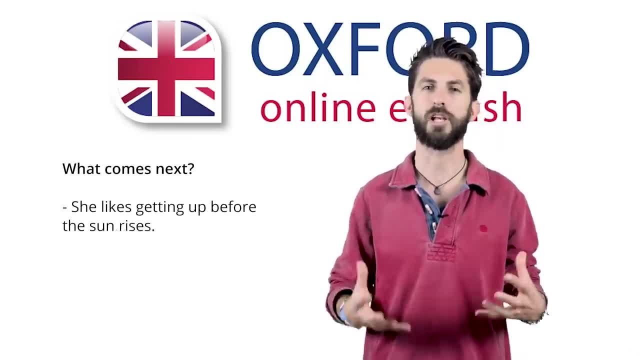 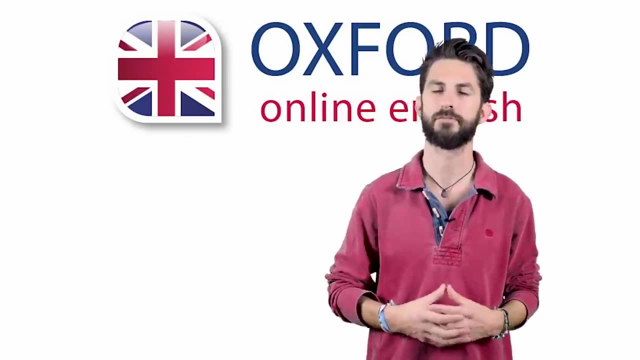 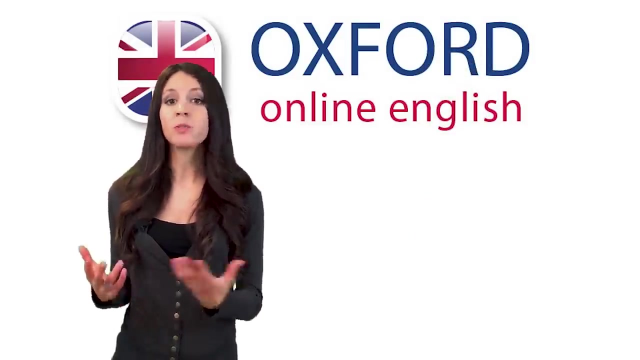 Before the sun does what She likes: getting up before the sun rises. OK, finally, we have a sentence which is both grammatically correct and which communicates meaning. What should you remember from this? Remember that when you use a particular word, you have limited choices in what kind of word you can use next. 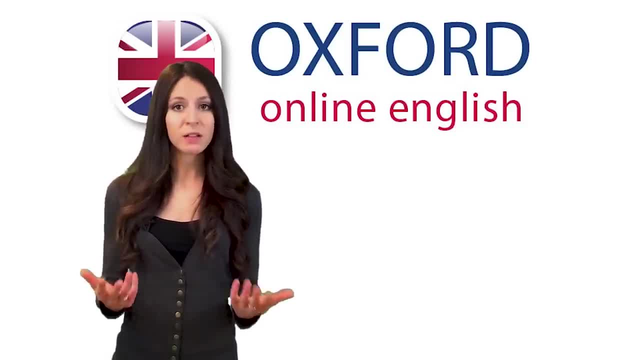 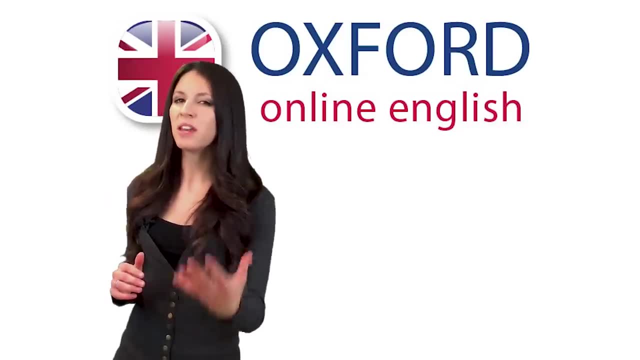 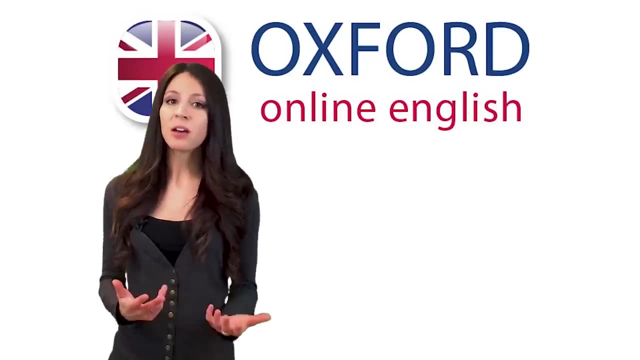 To speak or write in clear, correct English, you don't just need to know English words, You need to know what can come next. For example, with a verb like, like or want, it's not enough to know the verb, You also need to know whether the verb needs a complement. 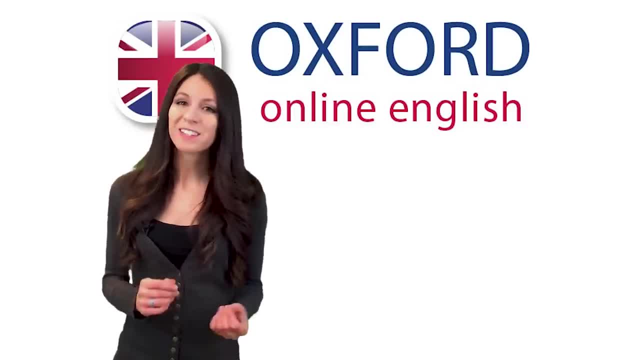 and what complements are or aren't possible. This is why it's good to learn vocabulary in full phrases and sentences. That way you'll know how to use the words you learn to make sentences you can use in your spoken or written sentences. 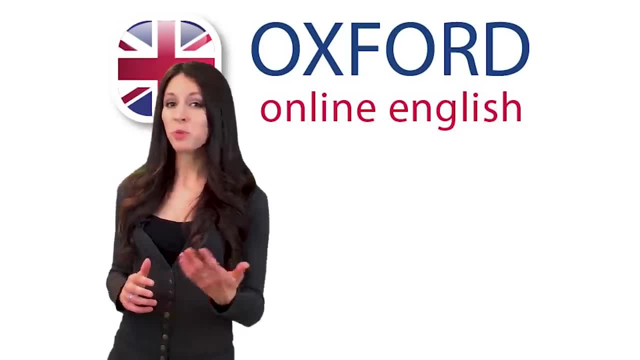 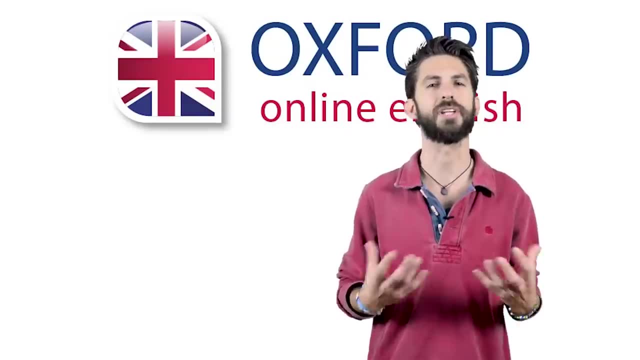 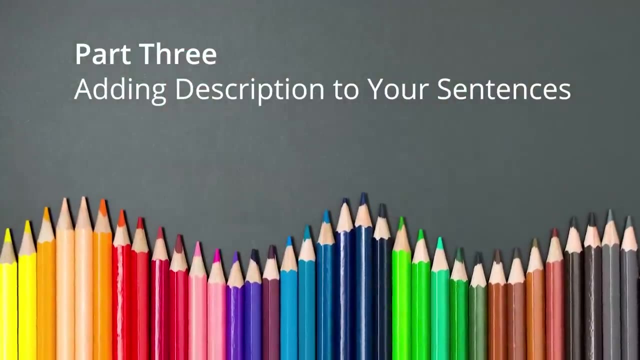 So let's take a look at a simple English sentence. Using what you've seen up to now, you can build many simple English sentences. Let's see how you can add more information and more detail to these simple sentences. You can add information to a simple sentence in two ways. 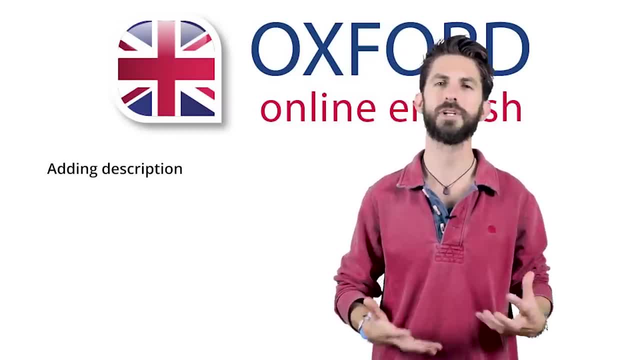 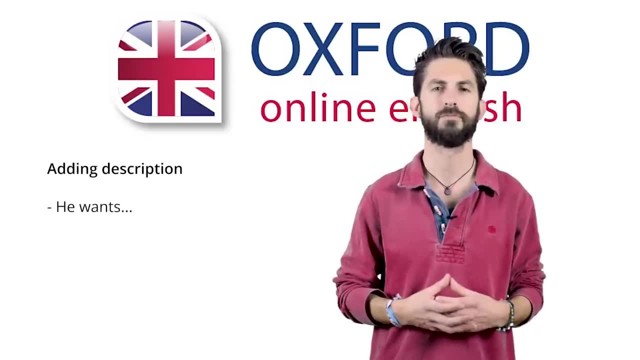 You can add adjectives or adverbs. You can add adjectives or adverbs, For example, using a sentence we started before but we didn't finish. He wants… Actually, you should do some work. Pause the video and finish this sentence in three different ways. 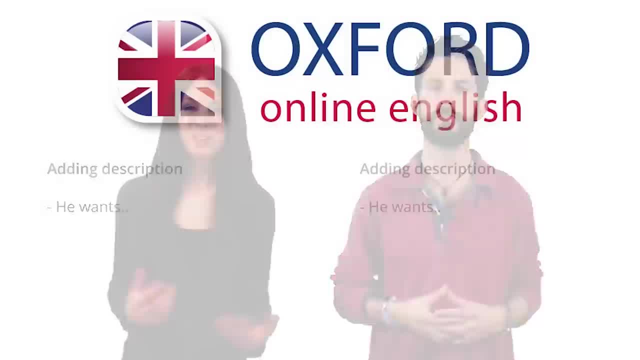 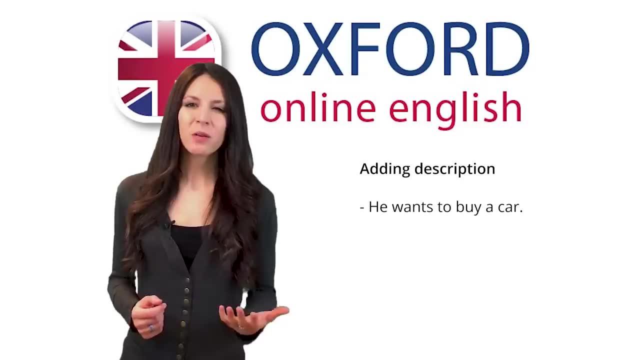 Start again when you have your answers Ready. Here's our suggestion. He wants to buy a car. Now let's add some description using adjectives and adverbs. Can you see how you could add adjectives to this sentence? You could add adjectives before the word car, like this: 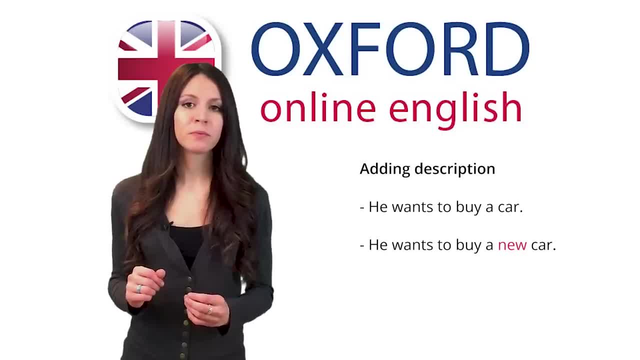 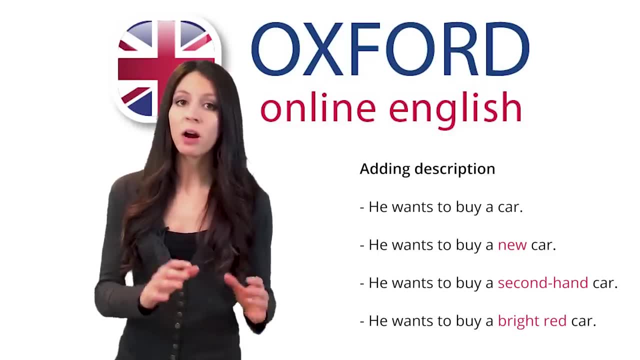 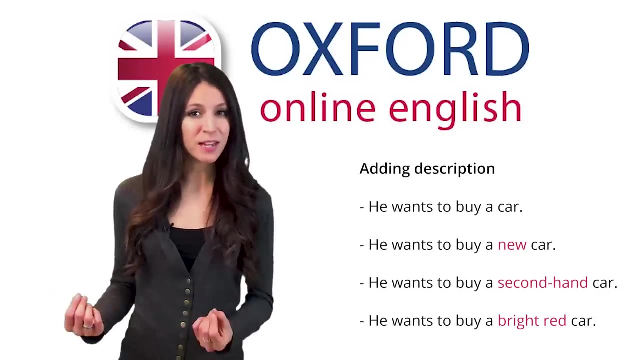 He wants to buy a new car. He wants to buy a second-hand car. He wants to buy a bright red car. What about adverbs? Could you add adverbs to these sentences to add some detail? Let's look at some of these details. 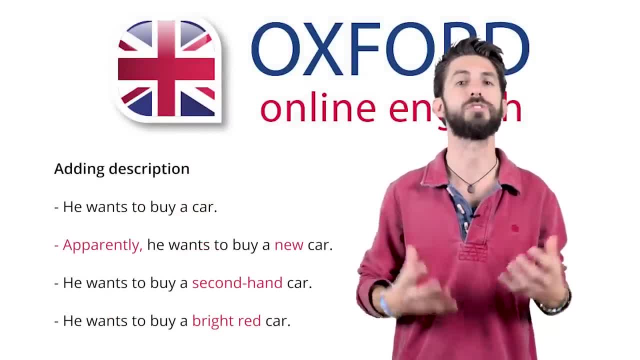 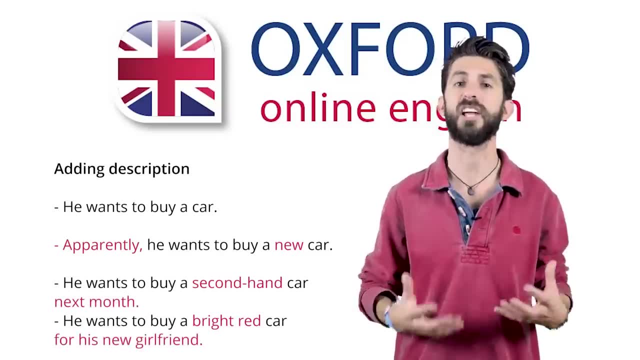 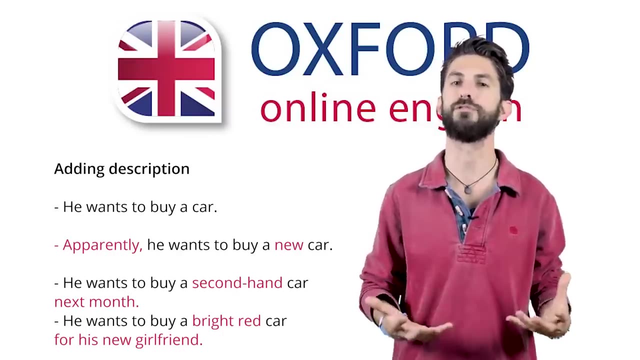 There are many possibilities. For example, Apparently he wants to buy a new car. He wants to buy a second-hand car. next month He wants to buy a bright red car for his new girlfriend. You can see that the adverbs can be single words or phrases. 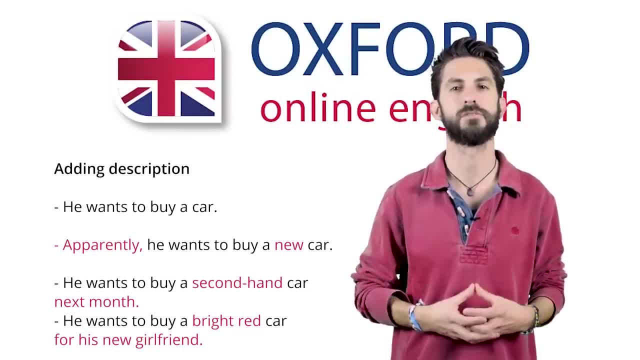 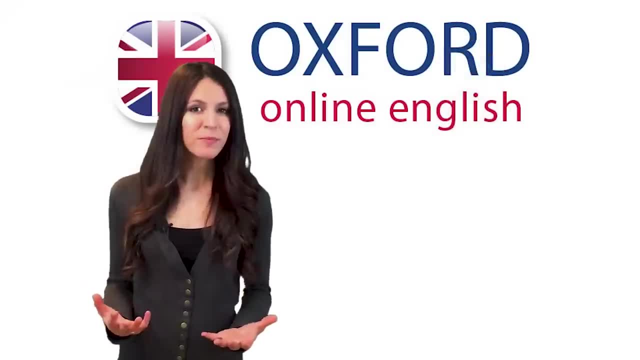 Adjectives can go before the noun they describe or after some verbs. Verbs are more complicated and can go in many different positions. However, this is the important point: Using adjectives and adverbs like this doesn't change whether a sentence is complete or not. 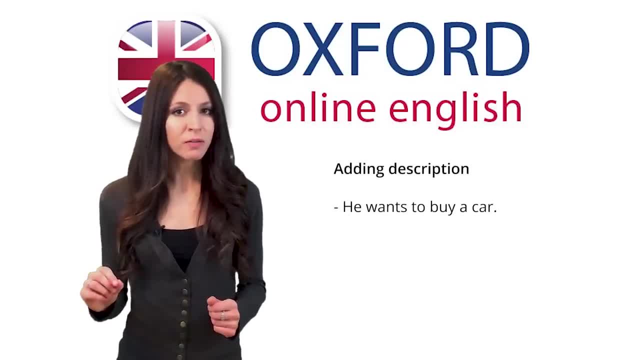 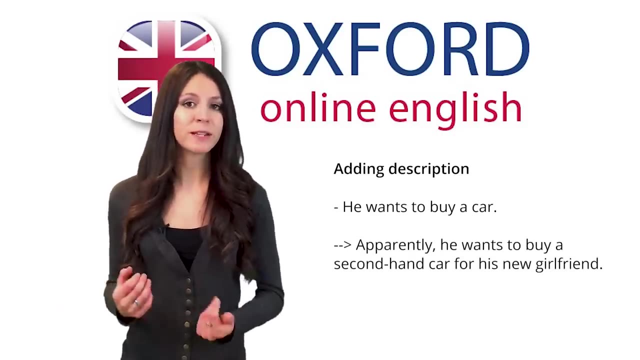 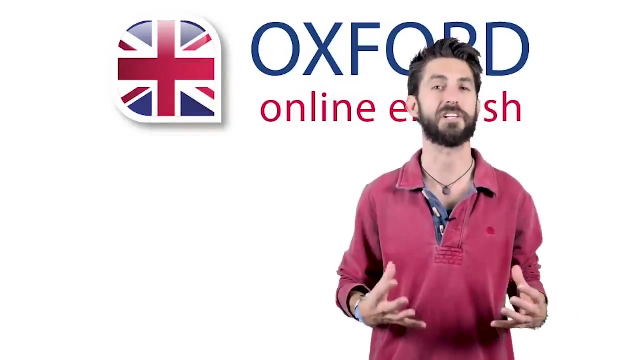 If you say he wants to buy a car, that's a complete sentence. You can add adjectives and adverbs to make it more detailed. Apparently, he wants to buy a second-hand car for his new girlfriend. However, if a sentence is incomplete, then you can't make it complete by adding adjectives or adverbs. 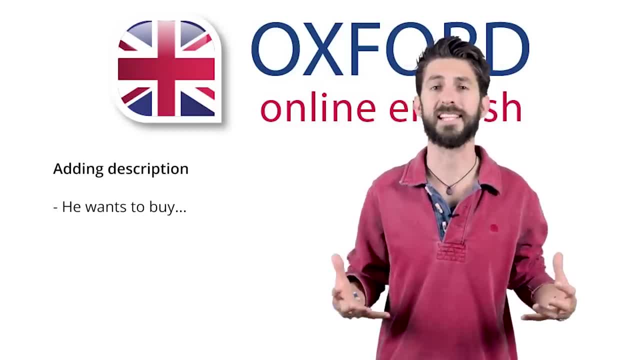 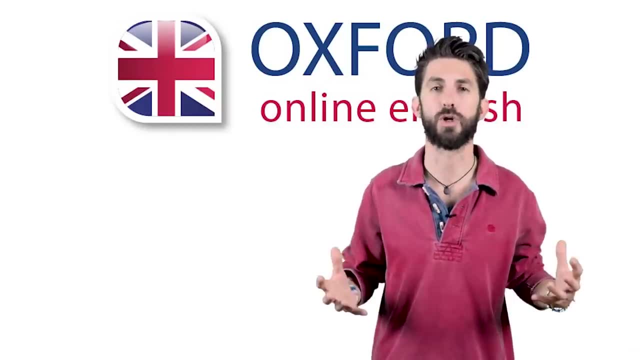 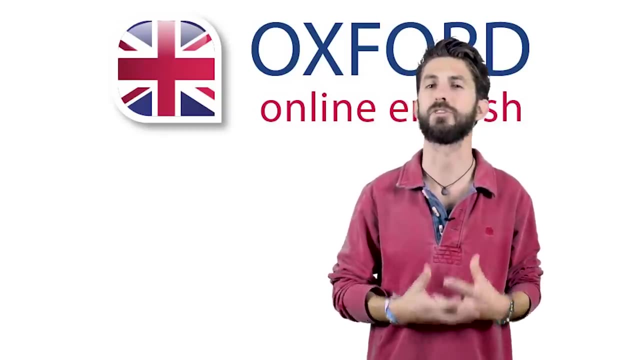 He wants to buy. This sentence is incomplete. Adding adjectives and adverbs won't make it complete, So at this point you can build a simple sentence. You also hopefully understand something about complements and why are they important for making complete sentences. 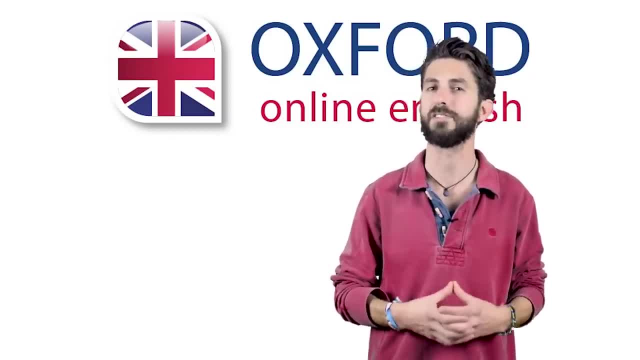 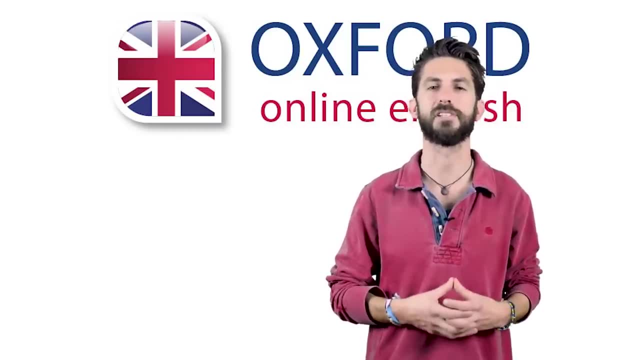 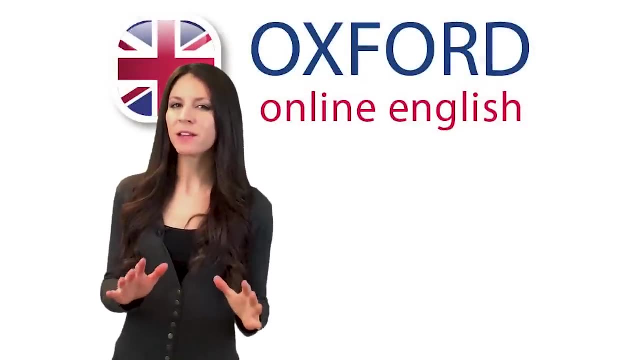 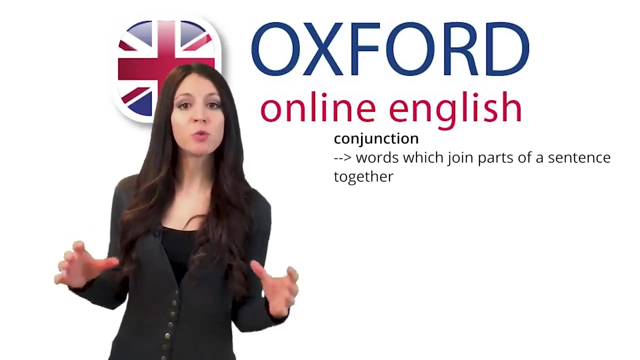 and now you can also add description to a complete sentence using adjectives and adverbs. Let's look at how you can combine these simple sentences into complex ones. First, let's define some words. A conjunction is something complex. A conjunction is something which joins two sentences or two parts of a sentence together. 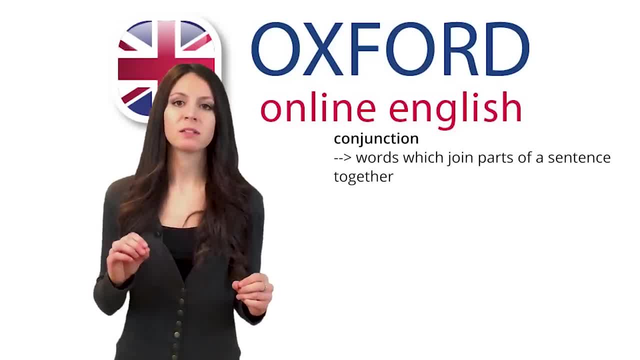 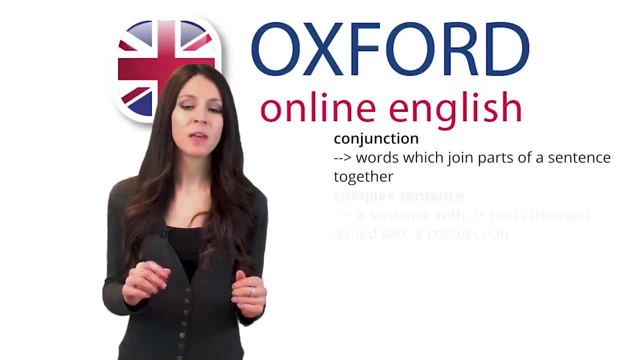 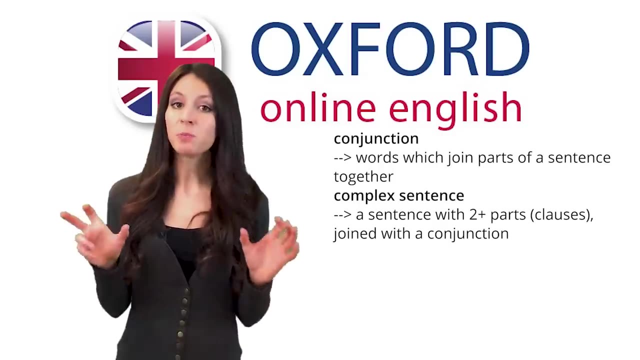 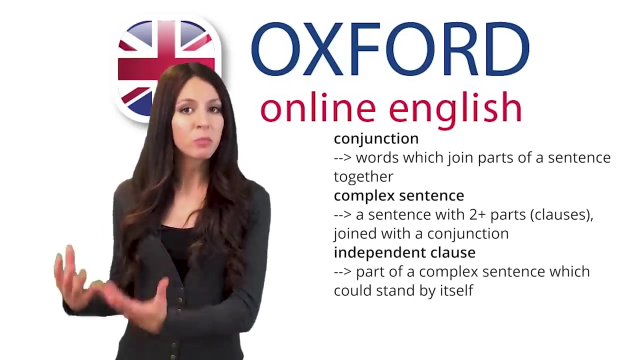 Words like and, but, if, although, because or which are conjunctions. A complex sentence contains two or more parts joined with a conjunction. These parts are called clauses. An independent clause Expresses a complete idea and could stand by itself. 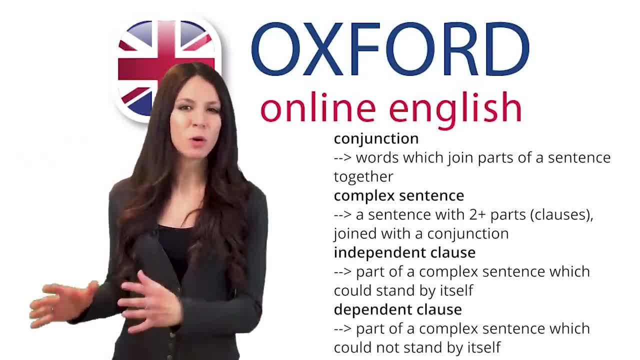 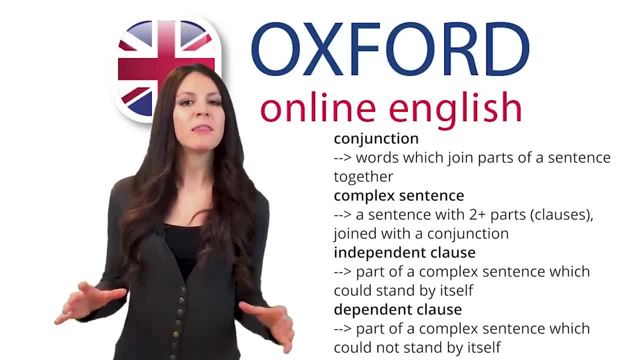 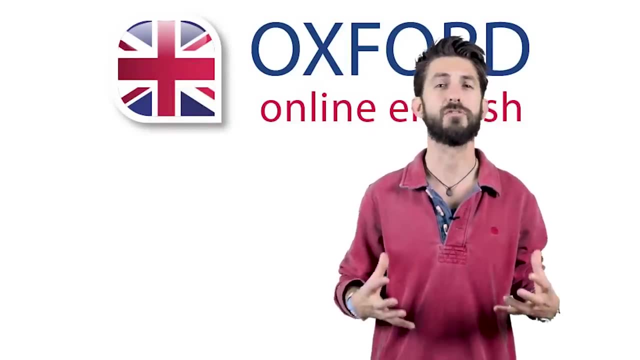 A dependent clause wouldn't make sense if it were by itself. A dependent clause depends on an independent clause in this same sentence in order to have meaning. Don't worry if this is new, You don't need to remember everything right now. 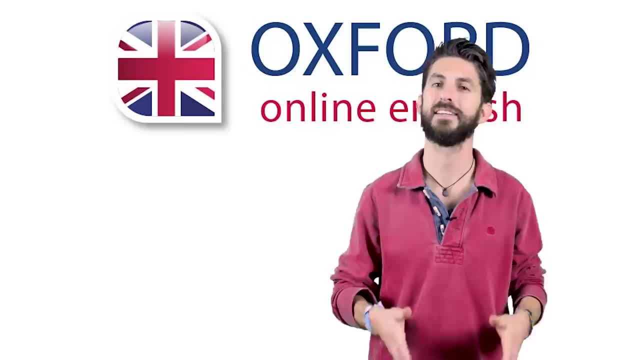 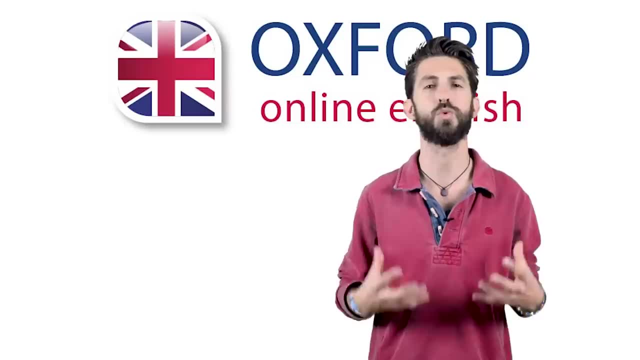 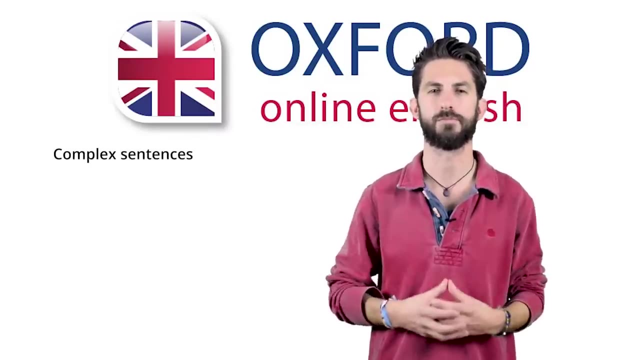 You'll see lots of examples of these ideas in this section and in the next section too. In this section, you're going to learn about complex sentences with two independent clauses. OK, enough abstract talk, Let's see some examples. He runs around the park every morning, so he's in pretty good shape. 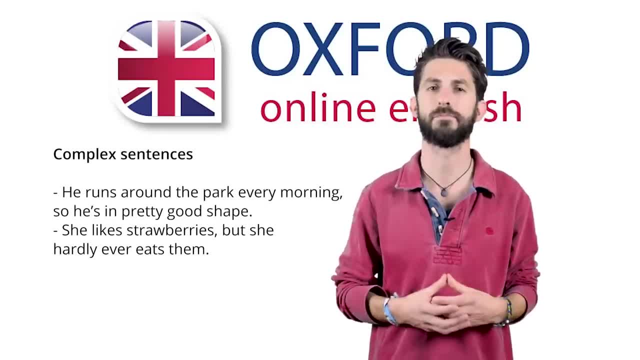 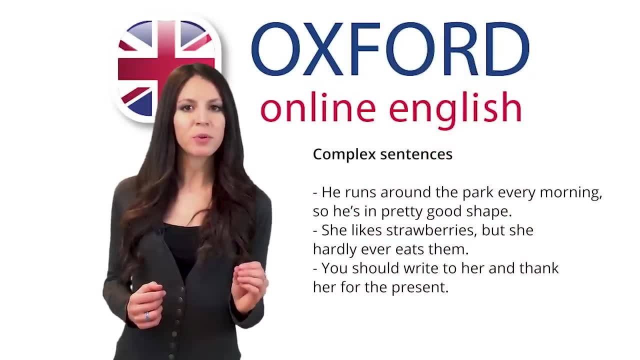 She likes strawberries, but she hardly ever eats them. You should write to her and thank her for the present. You should write to her and thank her for the present. You should write to her and thank her for the present. Here are some example of complex sentences. 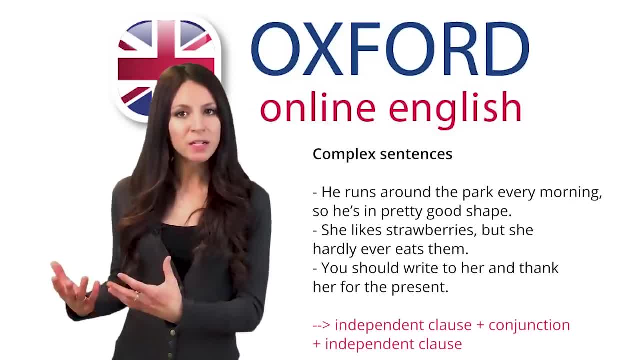 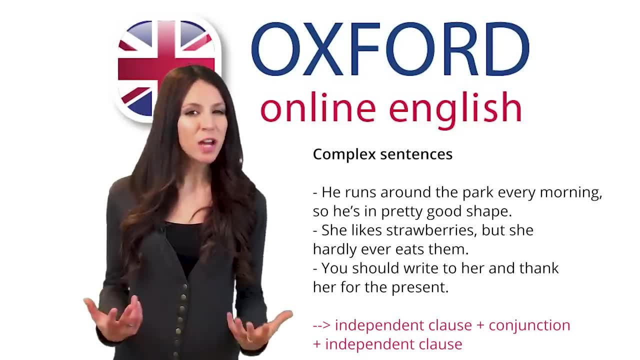 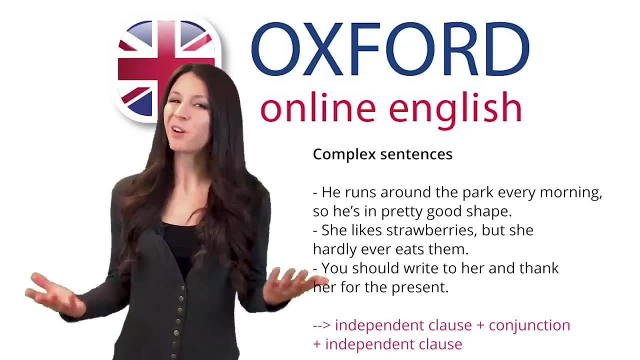 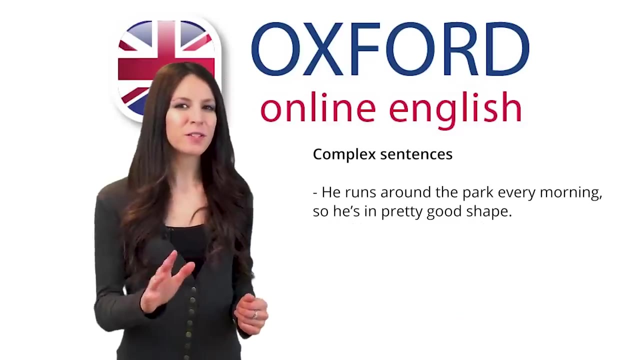 Here's your recipe: Independent clause plus conjunction plus independent clause. You generally need a comma at the end of the first clause, before the conjunction, But comma rules are quite flexible in English, so you won't always need a comma. Look at the first example. 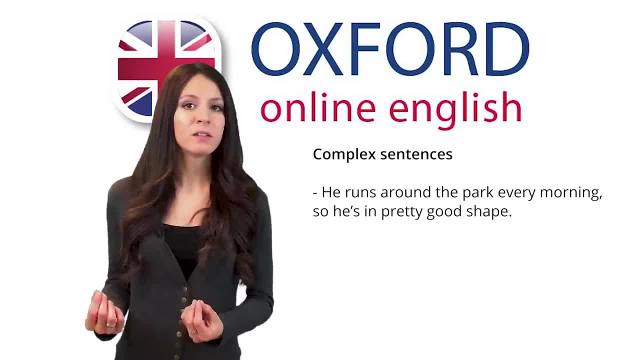 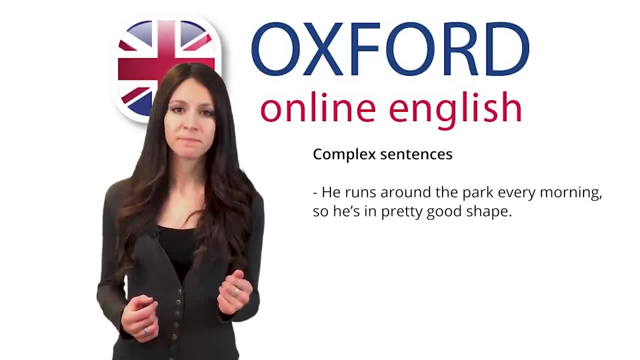 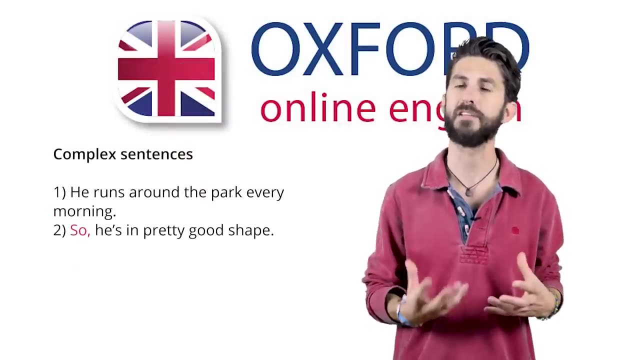 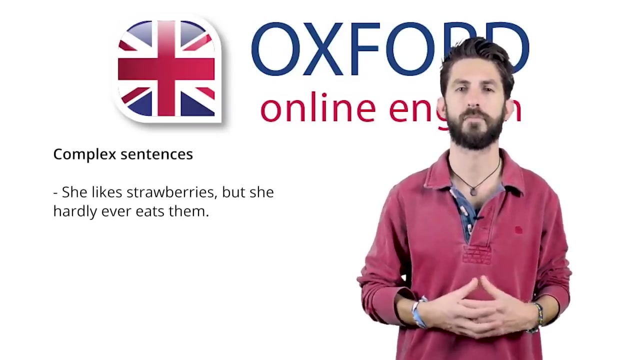 He runs around the park every morning, so he's in pretty good shape. Which word is the conjunction? The conjunction is so You can split this sentence into two full, meaningful sentences. Let's look at one more. She likes strawberries, but she hardly ever eats them. 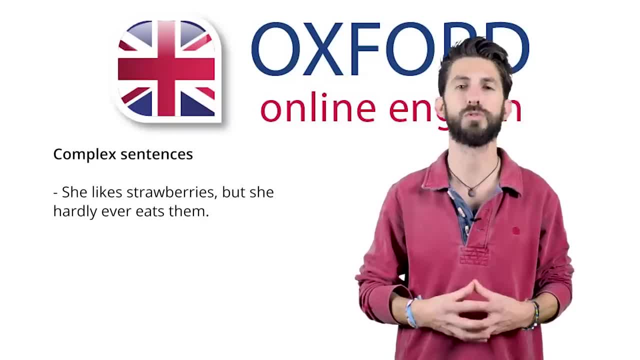 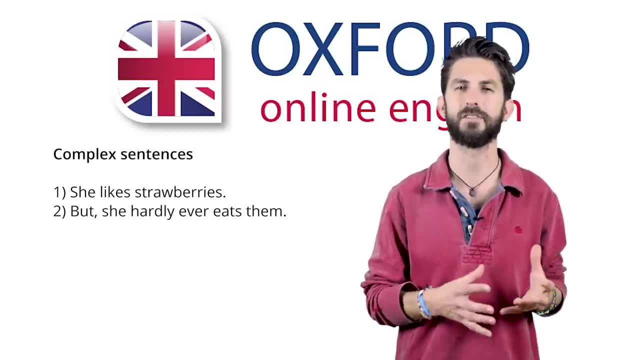 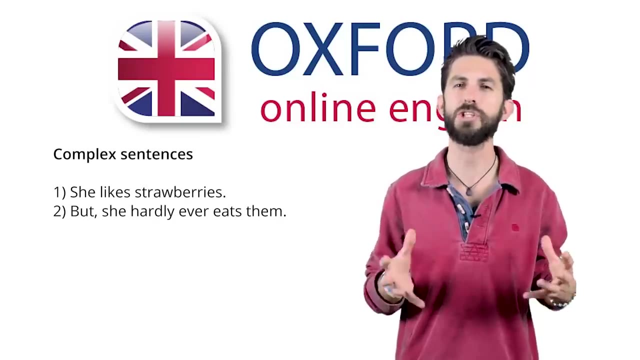 Again, you can split this into two full sentences. You might think that the second sentence here isn't complete or doesn't make sense by itself As it is. you'd be right. However, you can change them to strawberries and then it's a complete, meaningful sentence. 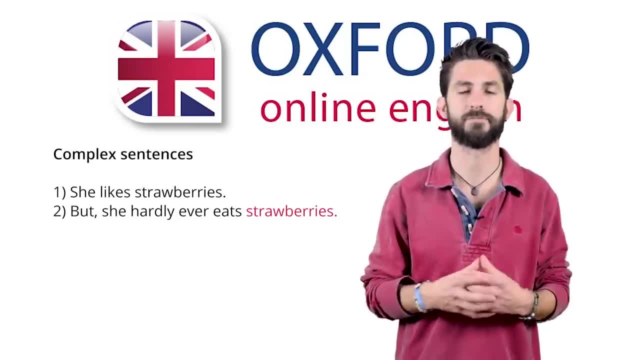 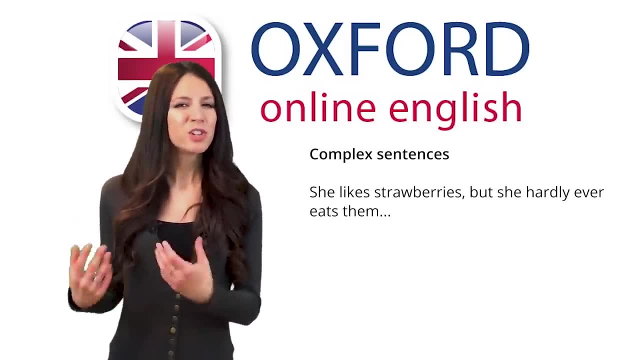 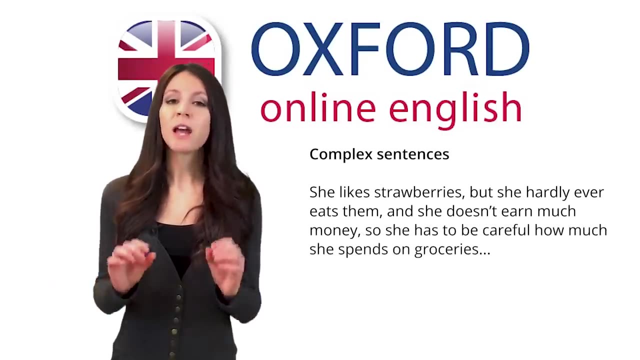 But she hardly ever eats strawberries. You can keep adding conjunctions and clauses. You can add phrases and clauses for as long as you want. She likes strawberries, but she hardly ever eats them And she doesn't earn much money, so she has to be careful how much she spends on groceries. 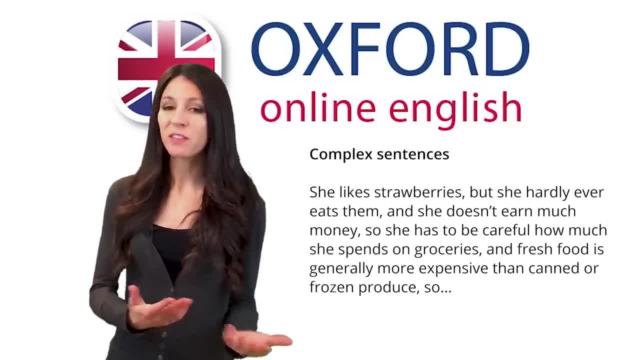 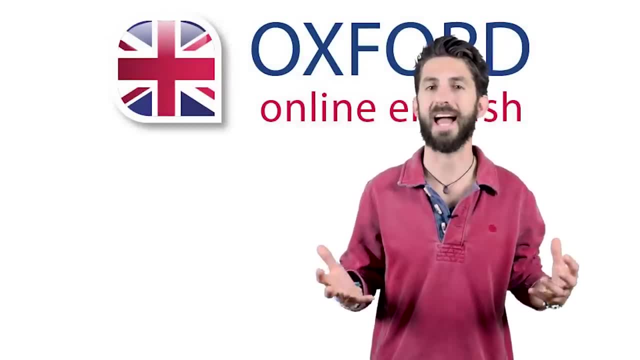 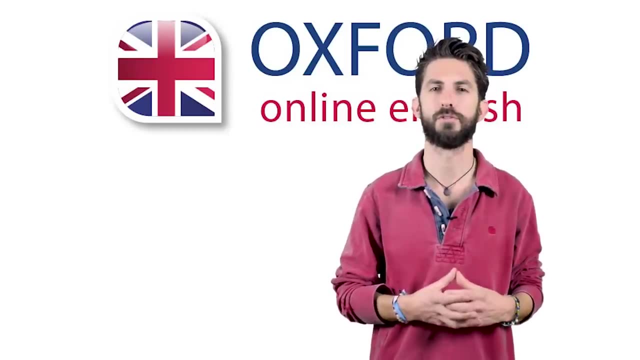 And fresh food is generally more expensive than canned or frozen produce, so …. Of course, just because you can, it doesn't mean it's a good idea. Sentences with too many clauses are difficult to follow, so it's generally better to limit. 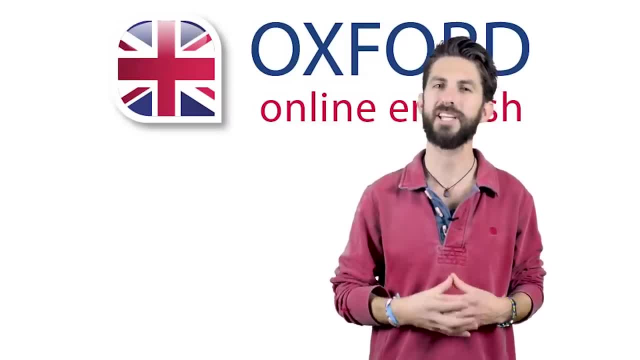 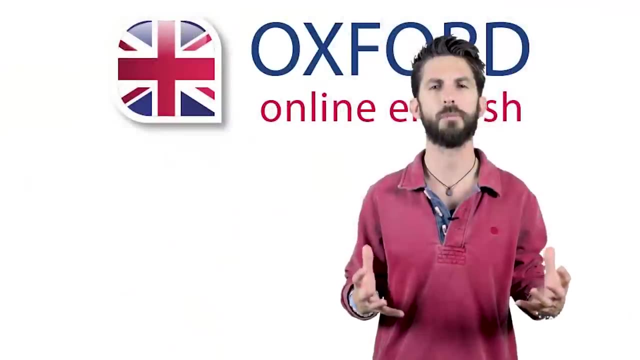 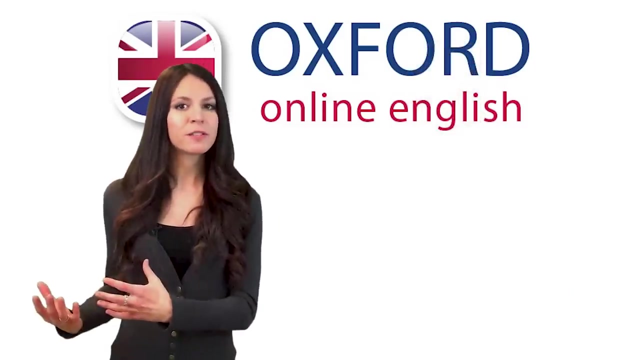 your complex sentences to two maximum three clauses. Now you know how to build a complex sentence using independent clauses. What about dependent clauses? Do you remember the definition of a dependent clause? A dependent clause is a part of a sentence which would not make sense by itself. 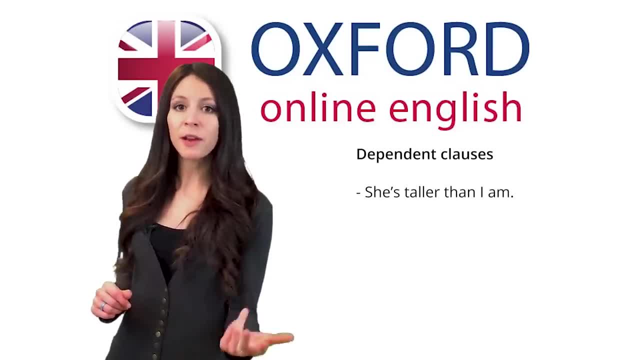 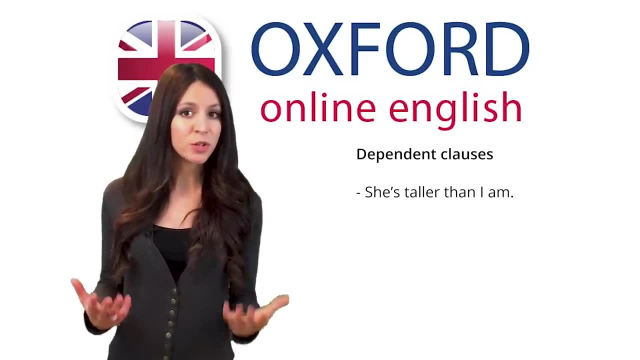 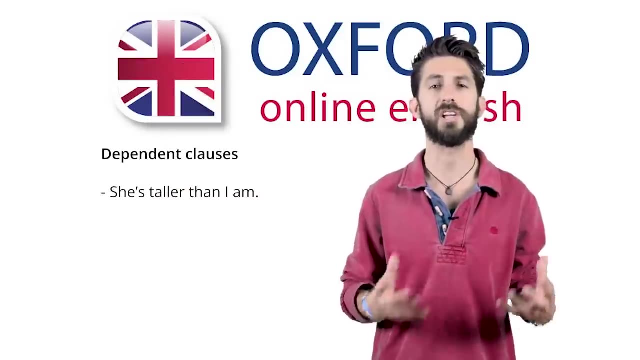 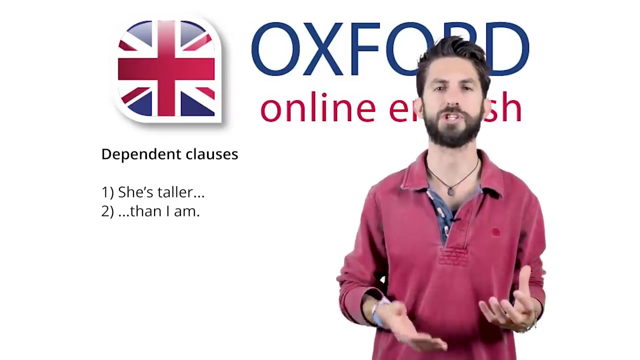 Let's see an example. She's taller than I am. This short sentence has two clauses. Can you see where the two clauses start and end and which one is dependent? The two clauses are she's taller than I am. They're linked with the conjunction than. 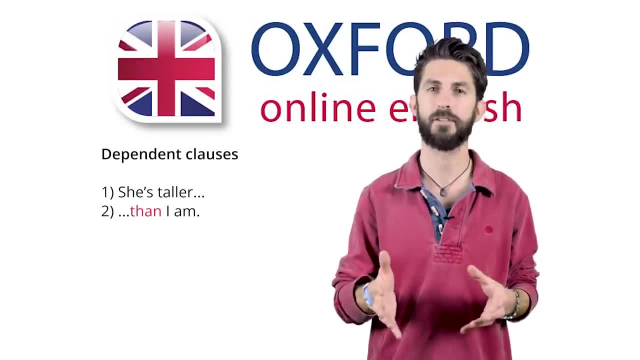 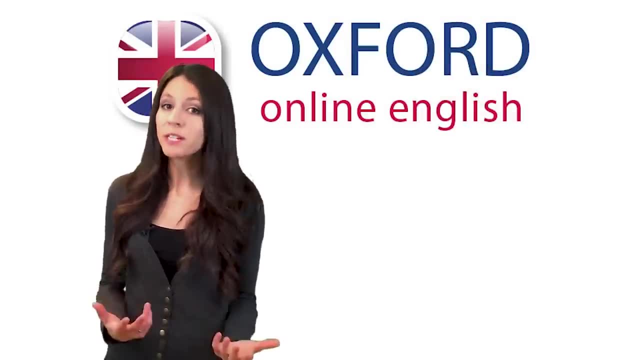 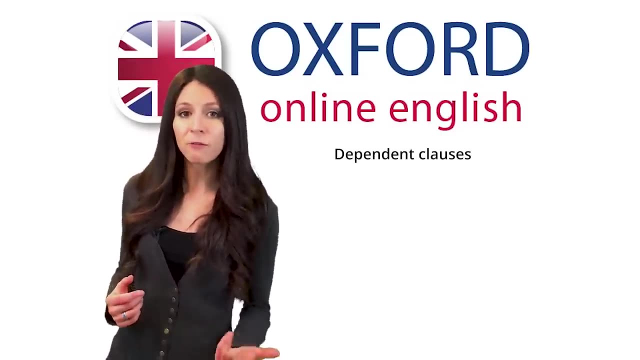 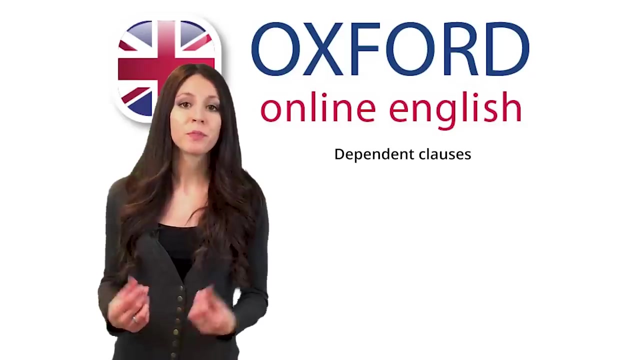 The second clause than I am is dependent. It doesn't make sense by itself. Let's see some other ways to build complex sentences with dependent clauses. You can add a dependent clause with conjunctions like if, because, although, unless or wherever. 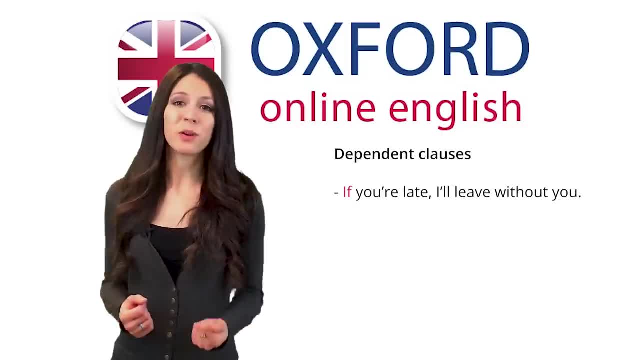 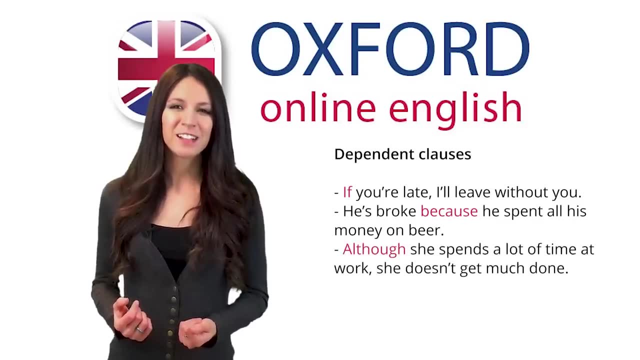 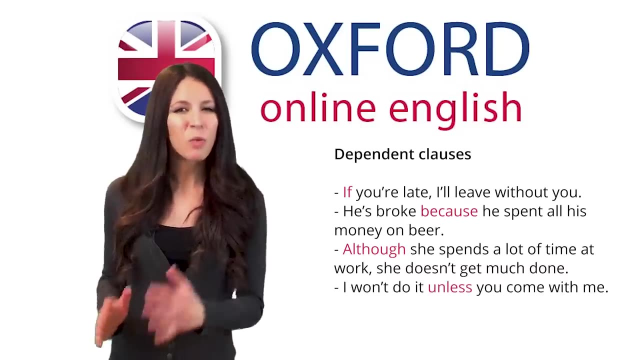 For example…. If you're late, I'll leave without you. He's broke because he spent all his money on beer. Although she spends a lot of time at work, she doesn't get much done. I won't do it unless you come with me. 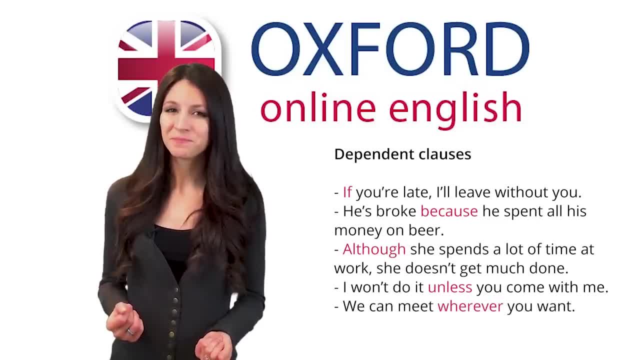 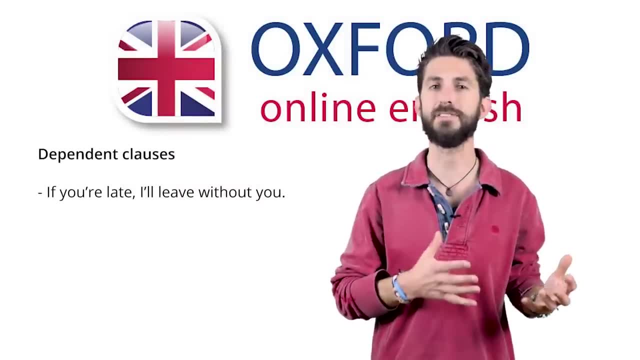 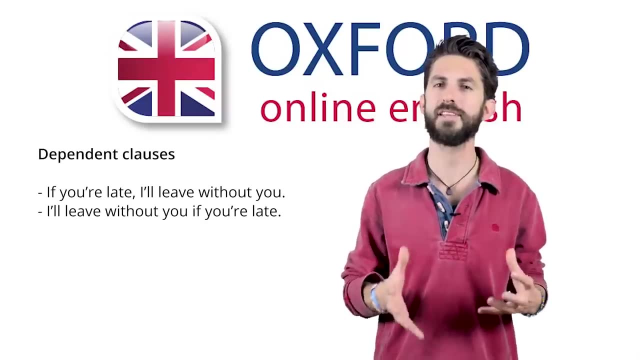 We can meet wherever you want. Often you can change the order of the two clauses if you want. So you can say: if you're late, I'll leave without you, or I'll leave without you if you're late. Notice that there's a comma between the two clauses. if the dependent clause is first. 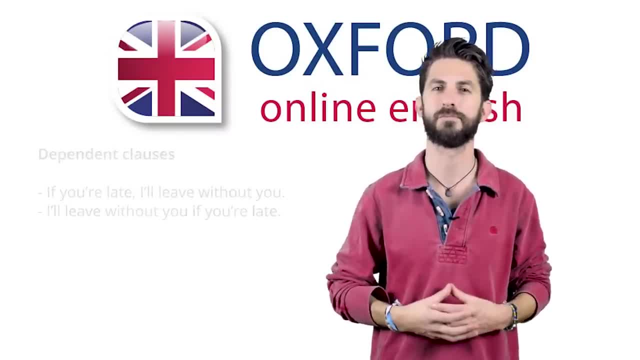 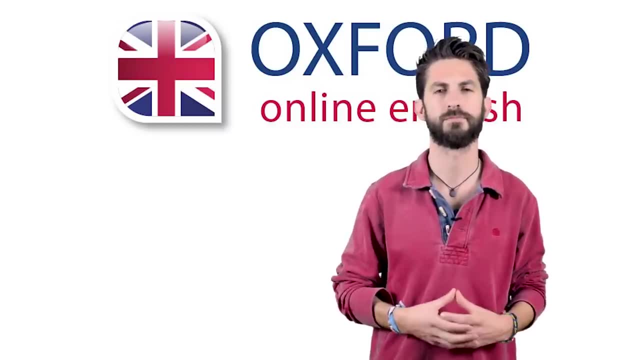 but not if the independent clause is first. What's the difference between these complex sentences and the ones you saw in part four? Here, you can't split the sentence in two. Well, you can, but you can't split the sentence in two. 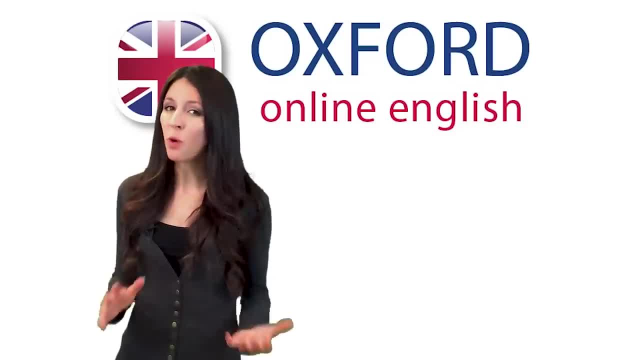 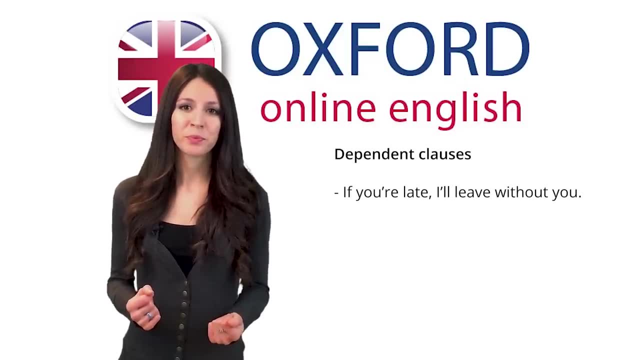 Here you can't split the sentence in two, But one of the two parts won't make sense. If you're late, I'll leave without you. I'll leave without you is an independent clause, so it makes sense by itself. But the other clause, if you're late- is dependent and it doesn't make sense by itself. 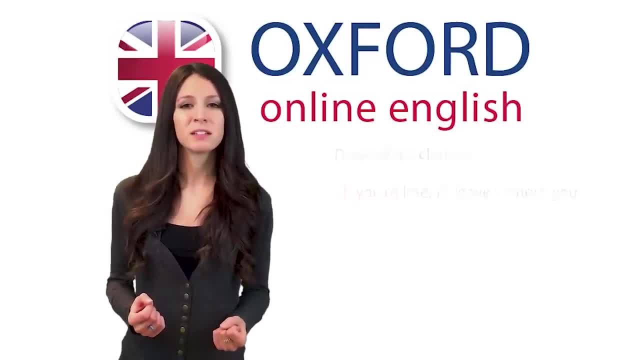 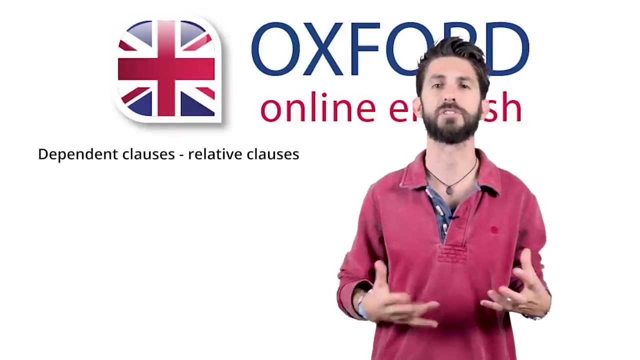 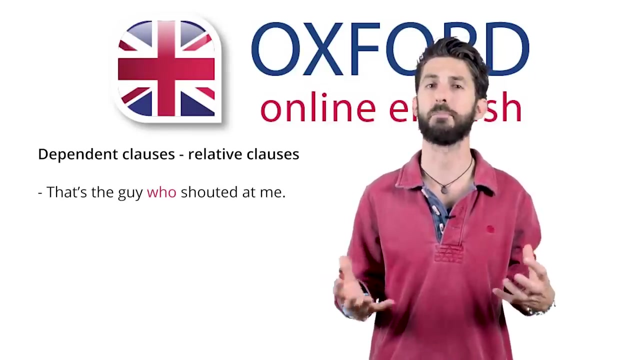 It needs something more to make it complete. What other common ways are there to build complex sentences with dependent clauses? Another common structure is relative clauses, using relative pronouns like who, which or what to link two clauses, For example. That's the guy who shouted at me. 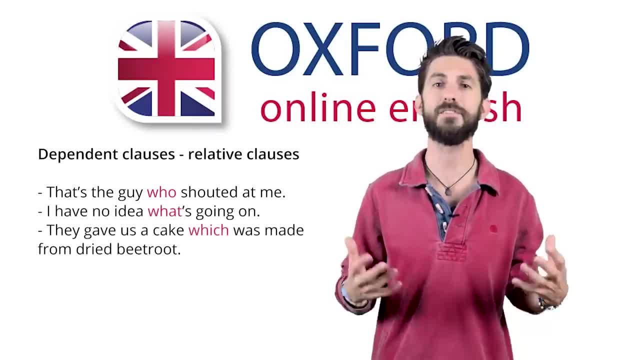 I have no idea what's going on. They gave us a cake which was made from dried beetroot. That's the guy who shouted at me: I have no idea what's going on. That's the guy who shouted at me: I have no idea what's going on.